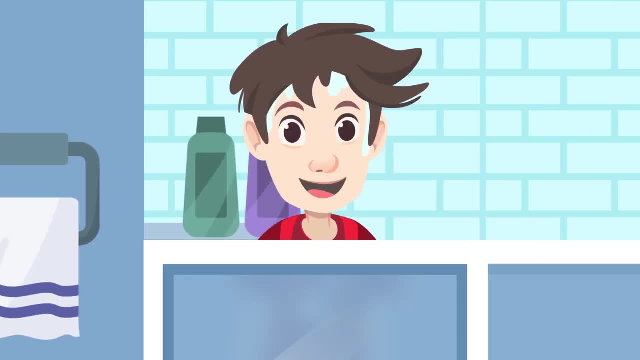 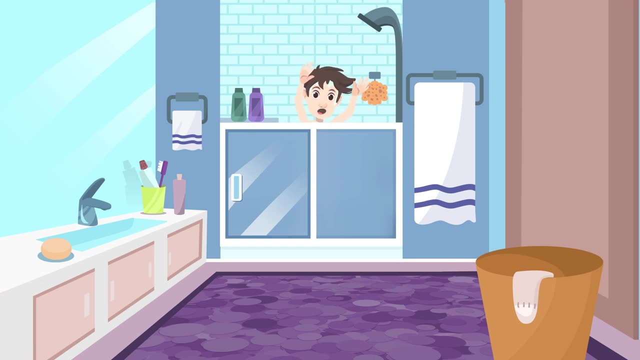 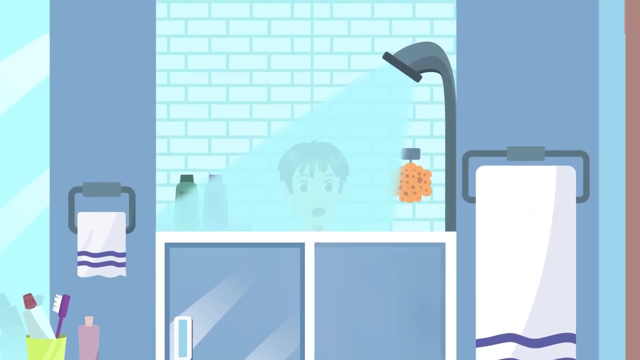 sports. I sweat quite a lot during the game and I'm going to have a good shower Now. we should toss the dirty clothes in the hamper. Three-point shot: Let's start washing our hair. We squeeze out some shampoo onto our palm. 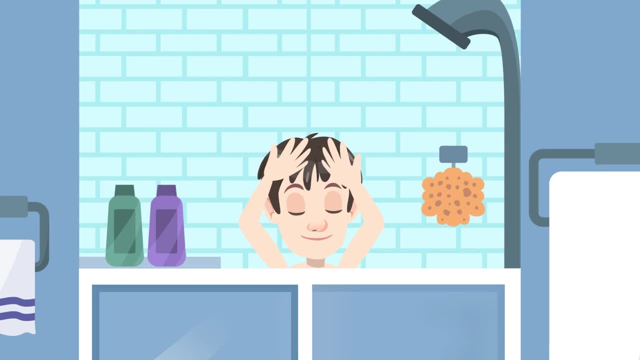 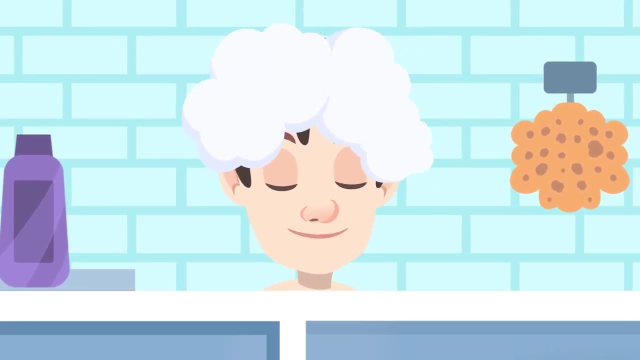 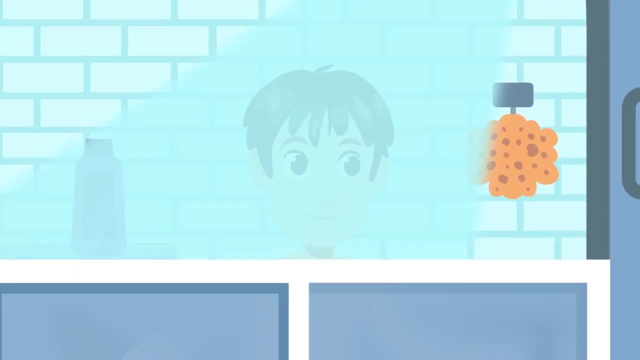 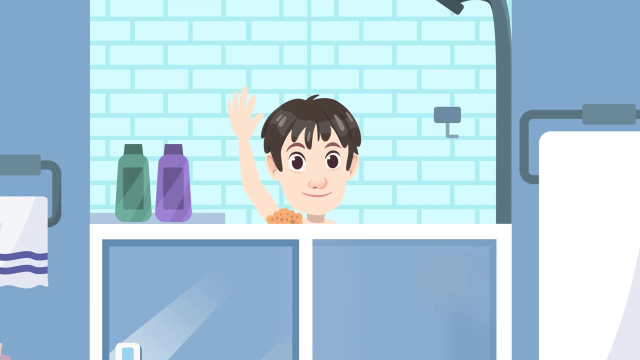 Foam it up. After a few seconds we rinse, Then we wash our body. It's best to apply a small amount of shower gel on the sponge and rub all over our body. Meanwhile we should turn off the tap to save water. 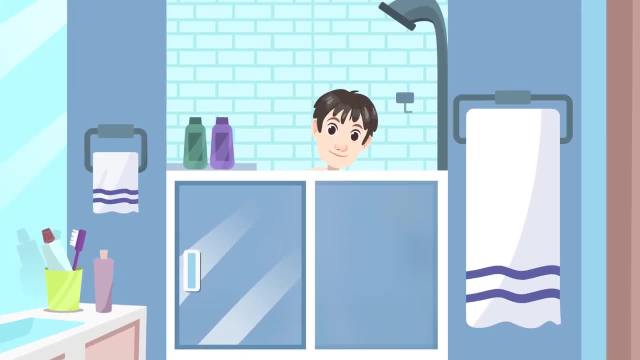 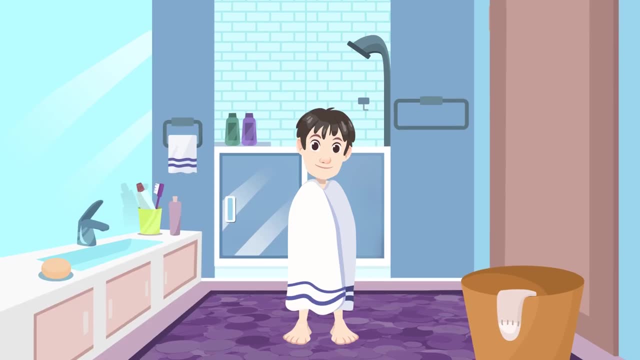 When we finish, we turn on the tap and wash our hair. I'm going to wash my hair. I'm going to wash my hair. I'm going to wash off the soap. I feel great after a shower. Now we should dry off with a clean, dry towel. 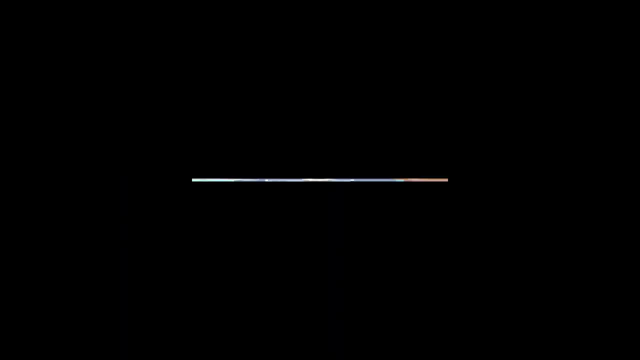 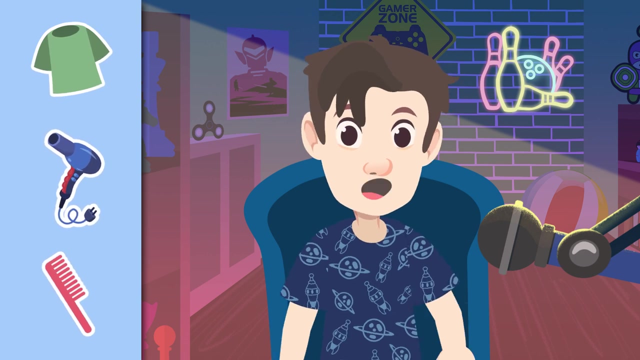 I'll see you in a bit. to keep talking about personal hygiene. Now I'm ready, I'm wearing clean clothes and I dried and combed my hair Much better, right? Another hygiene habit is to keep your fingernails short and clean. 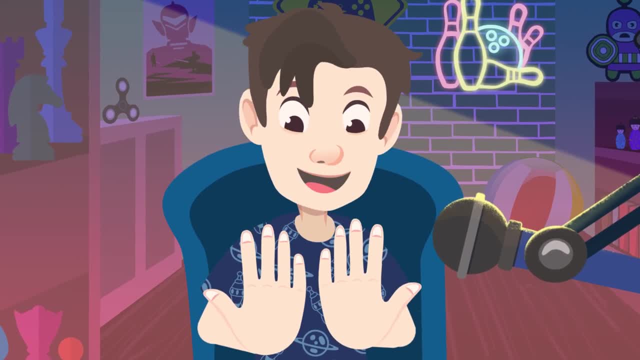 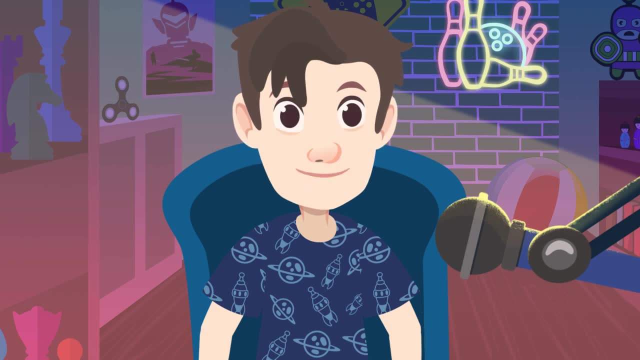 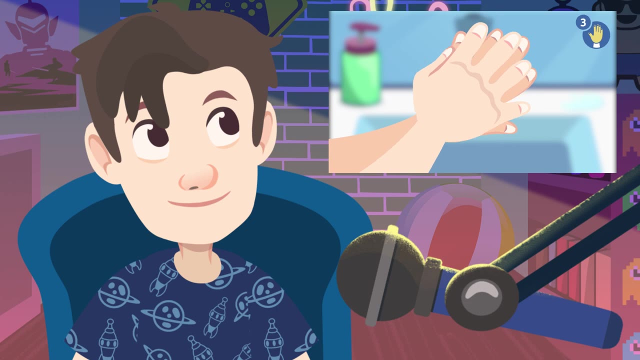 You should cut them if they are long, Using some scissors or a nail cutter. It's no good biting them. It's dinner time. They're calling me for dinner. I'll wash my hands well before sitting at the table. Learn how to do this watching the video Hand Washing on my channel. 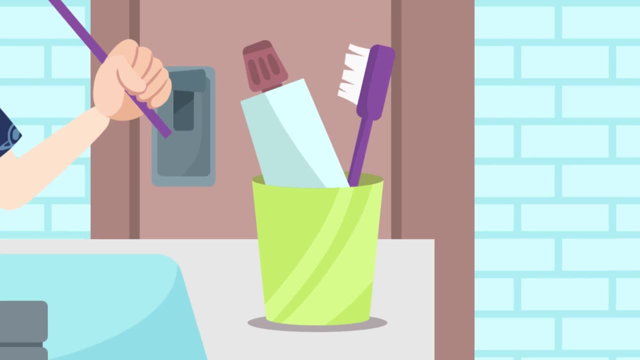 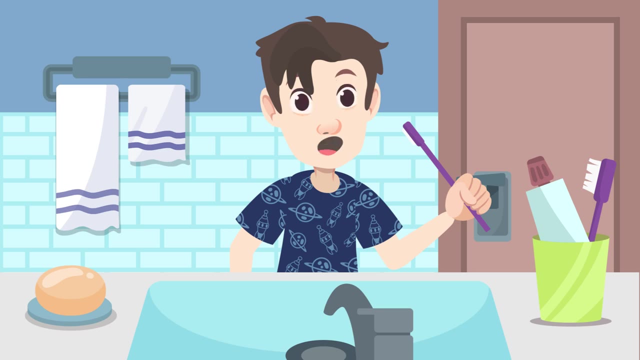 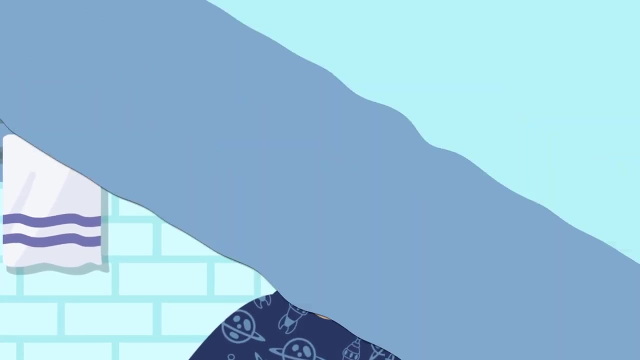 I'll be right back. Another hygiene habit is brushing your teeth after every meal. Brushing your teeth is an important part of your dental care routine and helps to prevent gum disease. The last hygiene habit we're going to talk about today is washing our face. 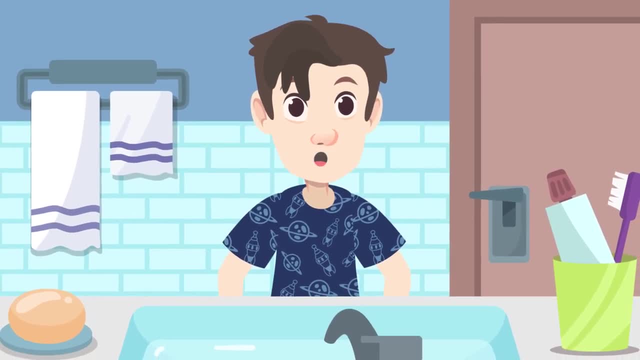 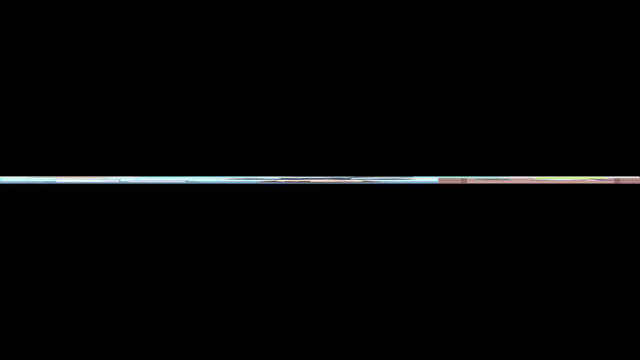 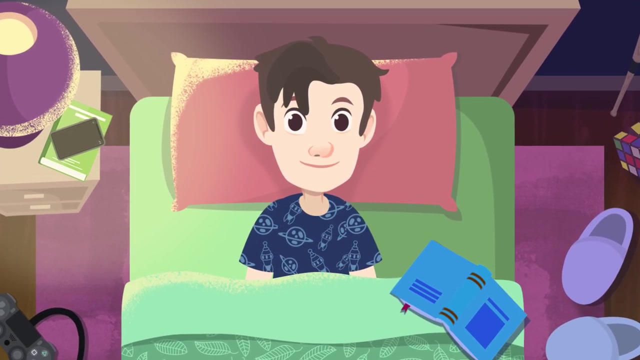 Before going to bed, we should wash our face. Oh, and in the morning, when we wake up, we should repeat this hygiene habit. I'm on it. What a day subscribers Want to recap the hygiene habits 1..